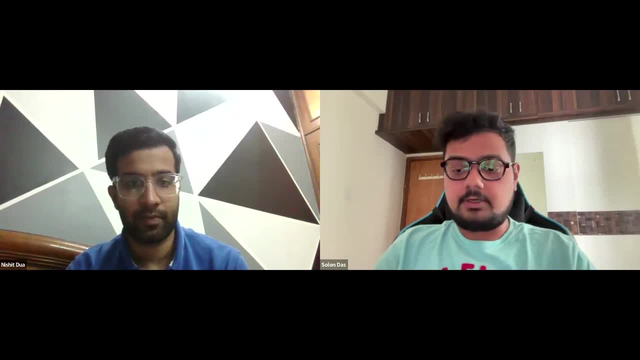 and Delta tables. Yeah, that's about it. You can start with your introduction. Yeah, sure, sure, Give a bit about the project that you are working on right now And like what use case you are solving and any challenges that you face on a daily basis. Sure, So I'm. 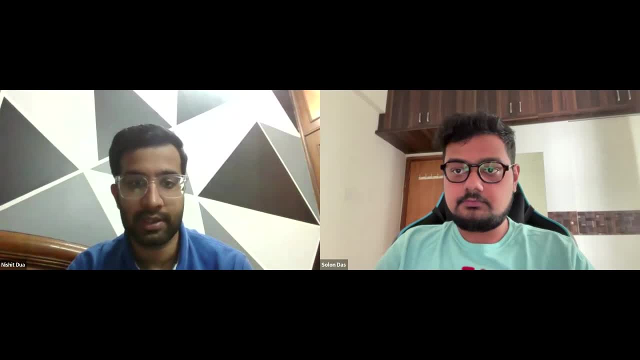 Nishant Dua. I graduated from Guru Gobind Singh Indra Prasad University, Delhi. Then I got an opportunity to work with Amazon as an intern. There, I started working on data tools such as Google Cloud Platform, And I also got to work on AWS and PySpark After that. since 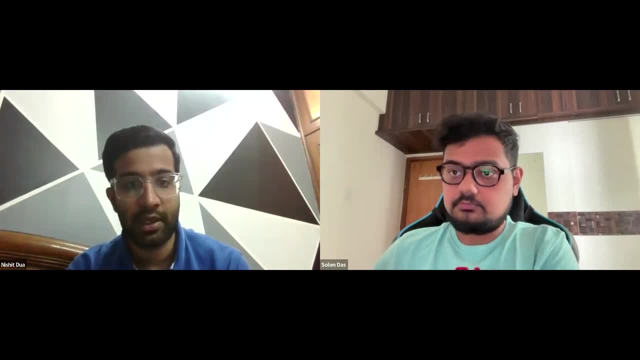 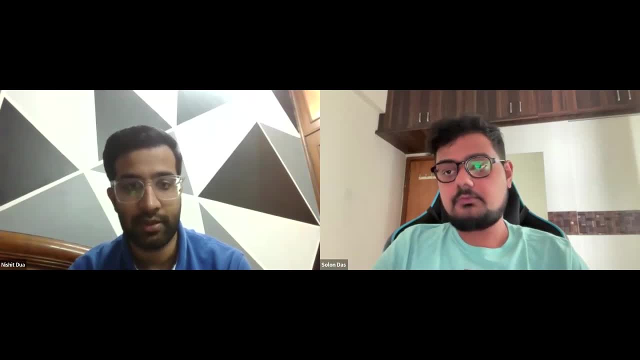 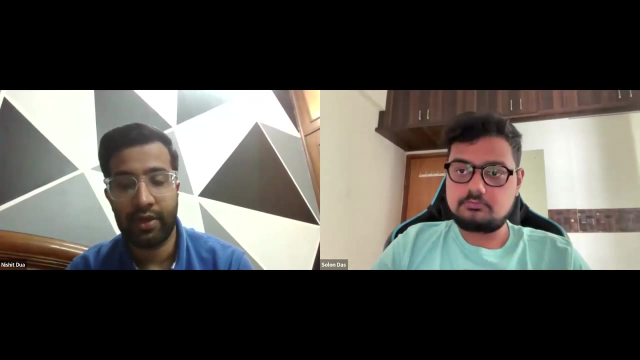 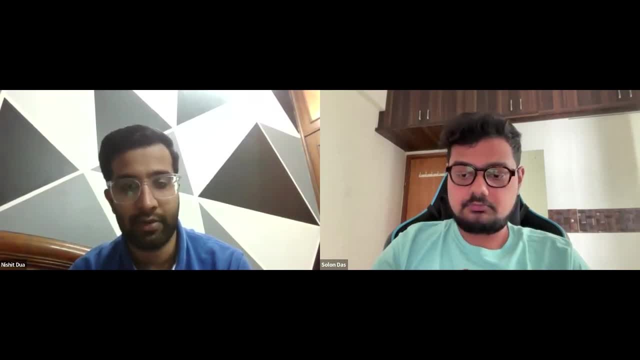 the tightping will be triggered every month. So earlier, what was the workflow business used to upload files from your website, or did you receive things in online version to the bucket and then we have to check it manually and trigger the tag, which was uh? 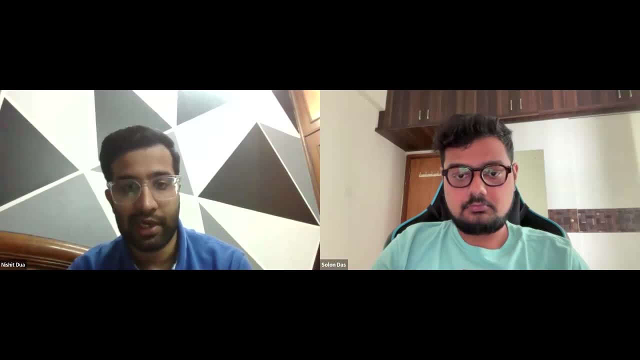 capable for to like validate the files for data quality. so, to overcome this manual process, what i paid was like i created a simple tag for a file watcher, so it will like we'll be triggering it, uh, for the first of every month and it would be triggered for, let's say, 10. 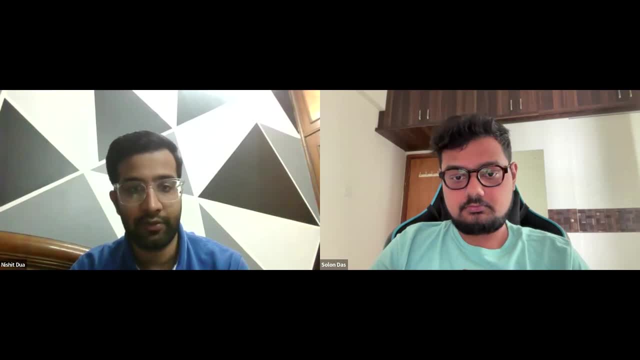 months and, if any, uh, in any time between first to 10 uh, when the file will be uploaded, then it will directly trigger the pre-evaluation load tag, which is, uh, like using trigger documentation. yeah, so uh, so suppose someone uploads a file after the 10th of the month, but then that? 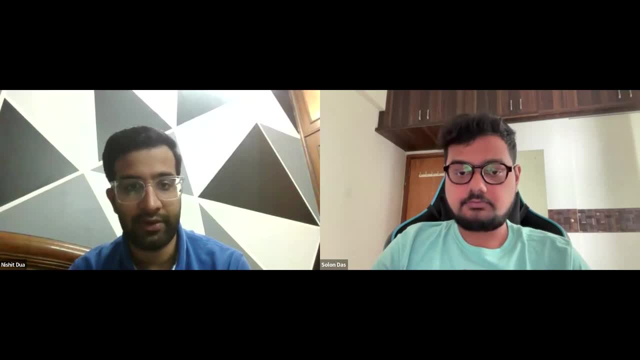 that would fail, like we were given it would be uploaded between five to seven, so we would just uh kept a buffer of three days. okay, got it, got it. um, okay. so uh, can you explain like in brief, like take one business use case that you solved. uh, i just want to get into. 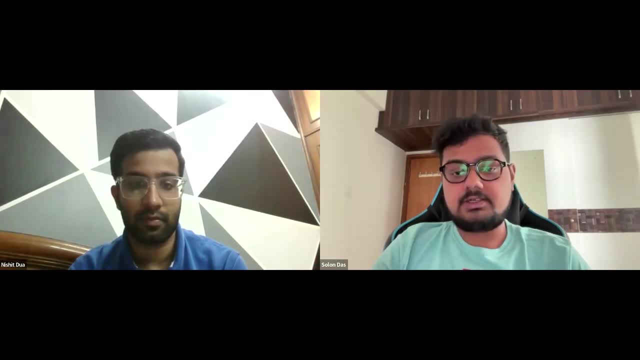 little bit more details about, uh, what was the use case that you solved for and, uh, how did you go about, you know, approaching uh the the de side, like the data engineering side? yeah, okay, so, like, as this project is new to me, so i'll like share my previous project, today's. 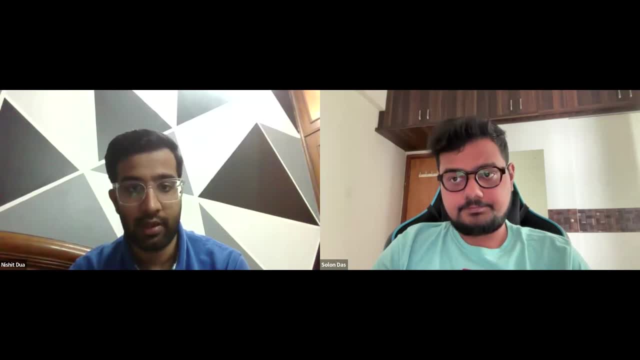 uh, there we had to work on a pharmacy data, so there we had a transactional data, uh, and we were using star schema, like there was a fact table which was having millions of record and it was also storing incremental data, and there was like, let's say, there were 50 or 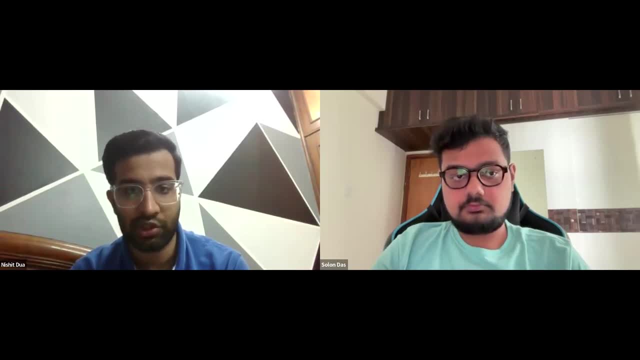 55 dimensions table which were linked to using the foreign key relationship. so that was the very first step in creating the same data with the fourth generation of the vaccine project. so what we faced is, uh, at start we were like when we were joining in spark code. 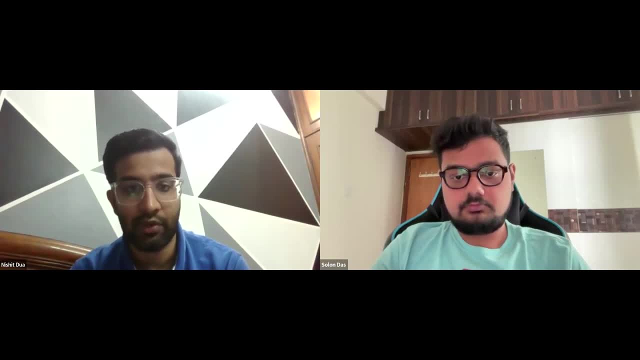 we were facing some delay. then we got to like we can use, as the size of dimension table was just in mbs for 2030 mb, while the fact table size was uh approaching to like 500, 600 gbs. so then we used broadcast joints for uh this. all the joints were joined in, so you. 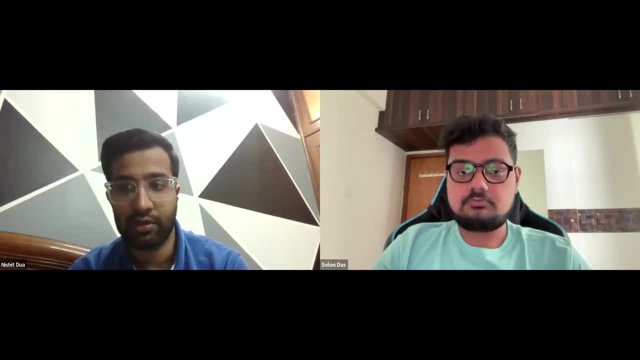 which we were doing on the fact table, so it reduced our like time from like i could say, 10 times. it reduced the time. so that helped a bit, so yeah, so, as you have already tapped into broadcast joints, so why does? why do you think broadcast joints when you do a joint between a smaller? 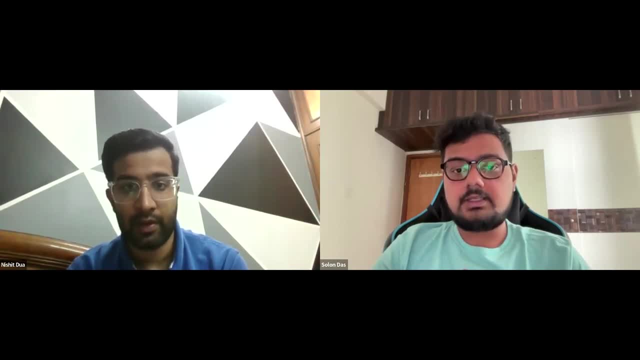 table and a larger table. why do you think broadcast joint takes a relatively lesser amount of time than a normal sort much join, sure? so let's take an example if we use normal join, so what would be like? all the data is present in partitions, so both the tables would be present in. 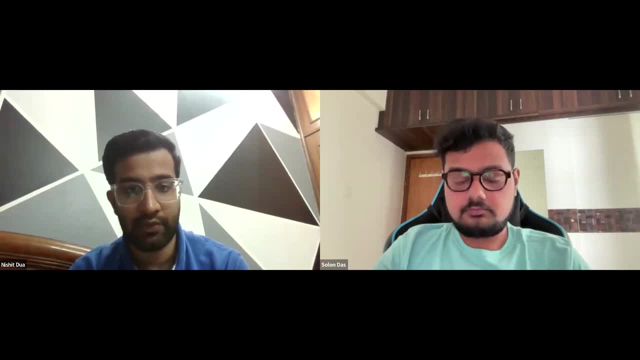 the partitions and like, let's say, if we want a join, which will be happening from data from one first partition to the third partition, the shuffling would be happening. so the shuffle operation makes like, takes a lot of time, while in the case of broadcast join, if the size of 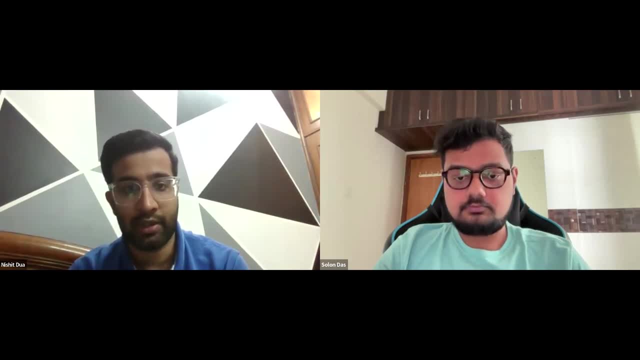 table is comparatively low that it could be stored in every node. then the shuffling operation would be not needed and hence it could take a lesser amount of time. okay, uh, just a quick feedback here. uh, so basically the broadcast table, the smaller table, is actually not present in each. 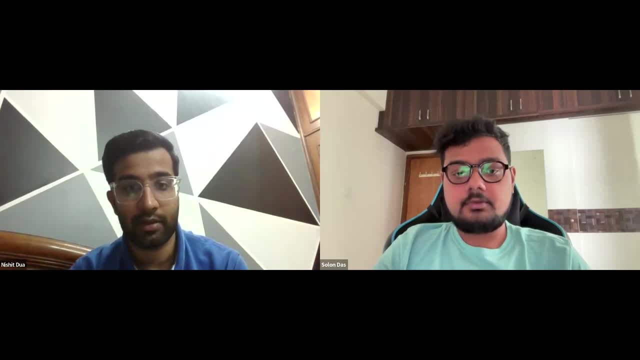 node. we are creating hash table for that. yeah, yeah, it's present in the driver table, casted to each node. yeah, got it. that's why it's faster and it reduces. it does not use shuffle, that's why it's faster. yeah, cool, uh, cool. so what are the other join types? do you know? uh, that helps us, uh, joining. 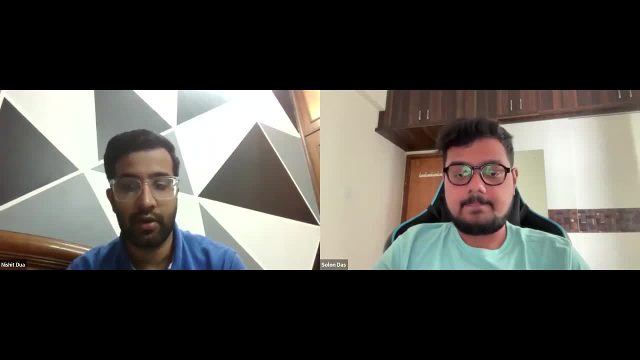 like two or more tables. one is shuffle, which is default. uh, also we can use- oh sorry, one is sort modes, which is default, and there is shuffle hash join that we can use in the cases where the data is large but not large enough to like. uh lot, not large enough to like it can be stored in partition. so there also like. 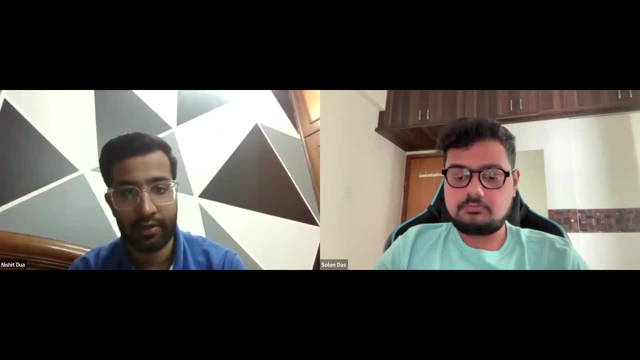 to some extent shuffling can be prevented. okay, okay, uh, can you explain partition tuning to me? uh, yeah, like let's say we are having some data which has been partitioned over, uh, four, let's say the partition number is four. let's say we uh apply some narrow transformation. so let's say, on our transmission, we just need. 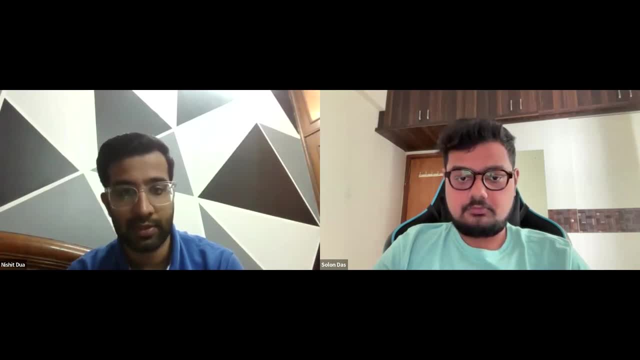 three partitions so we can just turn the next part, uh, the new, the partition which is has been vacant. that process is known as a partition phone, and how does this help? uh like, how does this help over a normal? so suppose you have a data set which is partitioned on a country? 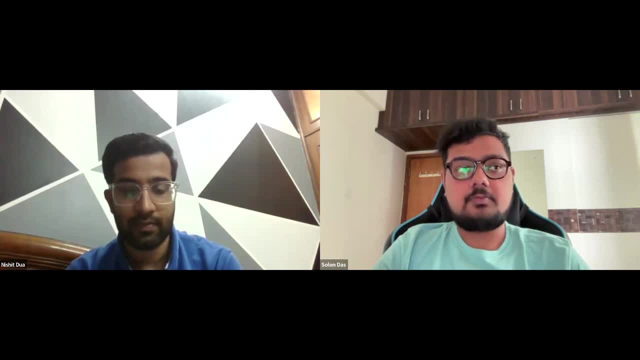 column- okay, and you have a data set which is partitioned on the country column. okay, and you have several other countries and you put a filter. so how does this help in reducing your perf, like, in reducing your time, uh, to get the result out and inherently optimizing your performance? 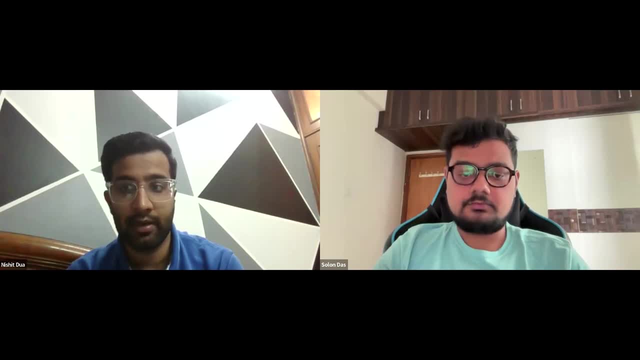 so first of all, it helps in memory management and when we filter our data on the partition column. so what is the first step? it will check all the partition indexes which are being created. so if we prune some partitions which are not in use, so the time would be saved there, like, let's say, we are. 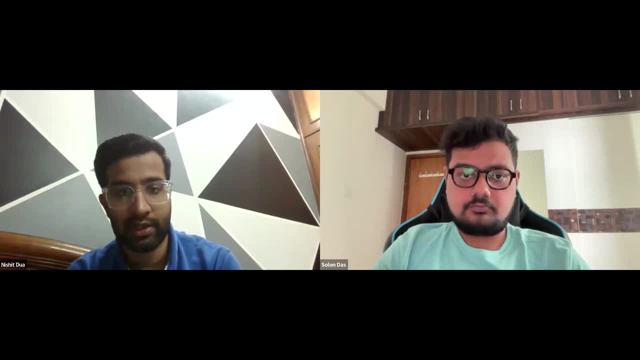 manually. uh, in the sql query we are manually checking uh under 10 columns which are like partition. so if we have pruned two or three columns it will reduce our time. okay, got it uh. so suppose there are 15 partitions, how many tasks would it create? uh, in the backend in spark. 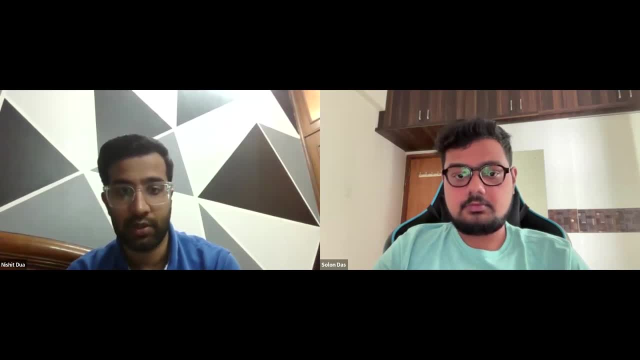 16, one for the driver node and one for each partition. yes, cool, uh. so, uh, do you know? can you explain a little bit about the principle of data locality? uh, i'm not aware of that. okay, uh, so it's basically, uh, keeping the data like not moving the data, and sending the code to the data so that we don't have to move the data. 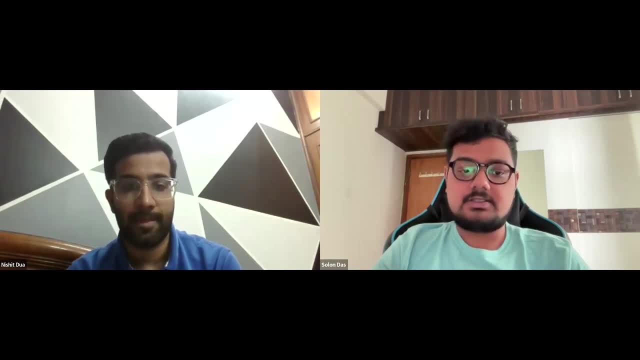 around. uh, this is what happens in a distributed system, like as we have multiple machines. we keep the data there and, as some shuffling you said, is an exp, expensive operation. we don't actually. we move the code to the data, to the machines, the operation is performed and this concept is known. 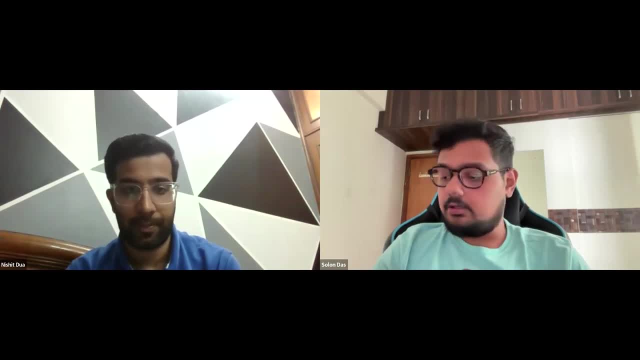 as principle of data locality. okay, uh, got it. so do you know about uh data storage levels? uh like, do you know what is serializing with the data posture of runtime and what is, uh the machine load costLES serialized? can you tell me the difference between serialized data storage level and? 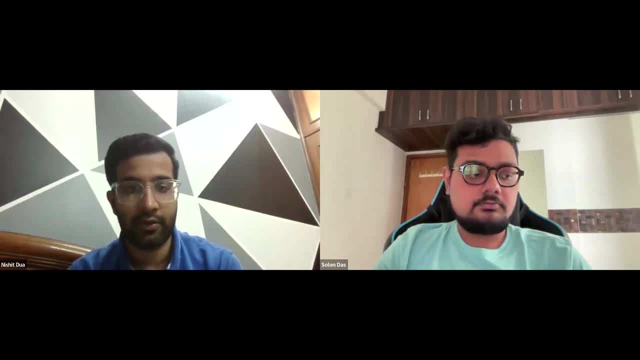 deserialized data storage level. so, like in the case of when we need to persist a data frame, we can just give our storage levels, which can either be memory. so if we pass memory only, so the cached data set would be only saved in the memory, while we can also use memory and disk so that it 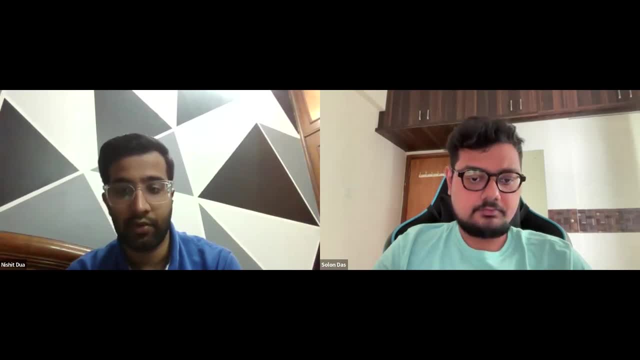 would be divided into memory and disk, like to reduce our memory storage. we can use memory only with serialization, so here we can save our memory so as it would be stored as a rdd which is serialized, but here a few like some time would be taken to deserialize the object. so it is kind of 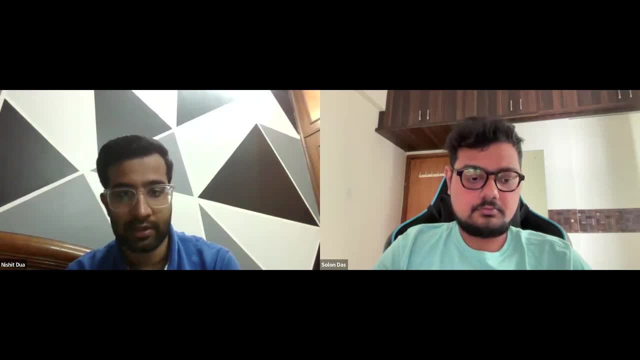 a trade-off. if you want to reduce a memory, we can just take some extra time to deserialize and serialize and and and. which one of them takes more like? which one of them provides you more amount of compression for serialized? serialized, okay. do you know the different read and write modes that we have? 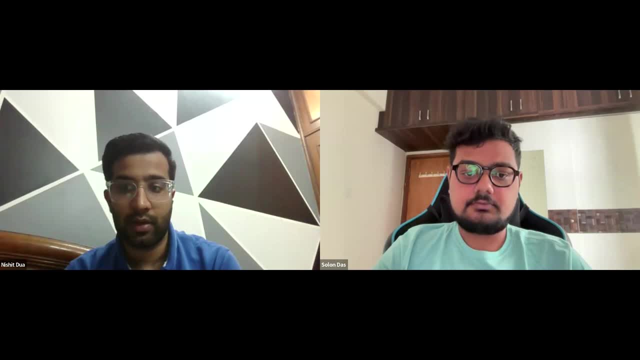 for our data frame reader and writer, api. we can, in read mode, we can choose format and it would be like we can pass any format like csv, json, text file. no, no, not the file format. so so the reading modes, like we have permissive. so in that grounds i'm saying so, basically, writer. 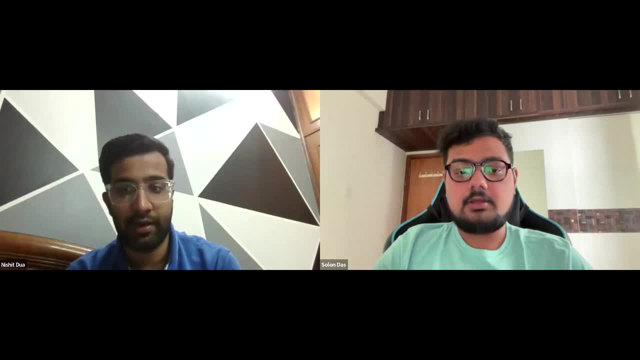 modes. if i say, whatever we can use, append, overwrite, but like if we have incremental data, so we can just append that, append the data frame, so the incremental data is loaded into the target table, like if we want to, uh say, overwrite it so we can use it, the earlier data would be in this function. 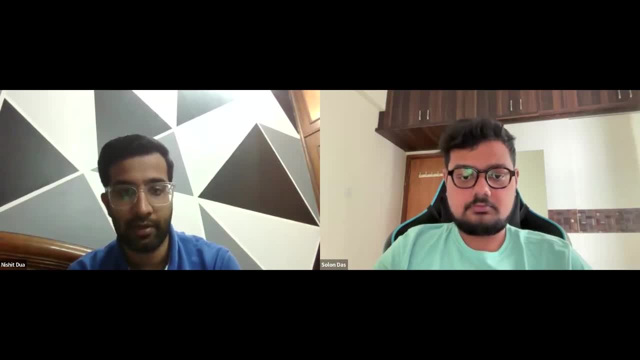 be truncated and the new data would be loaded in the table. okay, so how do so suppose you're appending a data set, so you are doing an incremental load every day. it's a refresh that is happening. how do you ensure that the data that is coming along every day is not the same data? 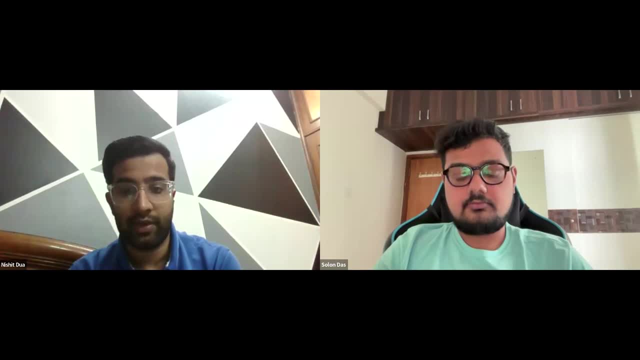 that is already existing. for that we should also be reading that red target table and we can perform a left anti-join on that data and to fetch all the new records which are being present and that are not duplicated, then the targeted data frame. we can use append mode to write it to. 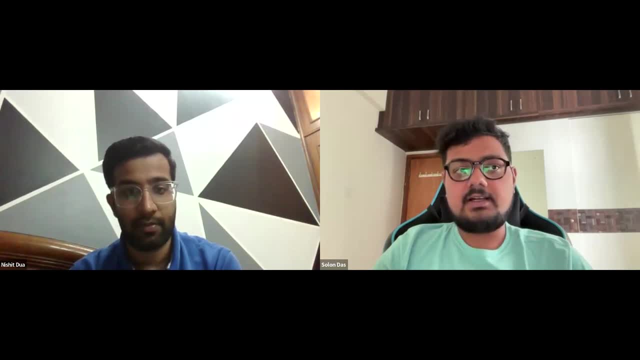 the data or table. so your left anti-join will be performed under like what scenario, like what would be your column combination like: do you check it, check the left anti-join- with the whole row as such, or do you do a like with a certain set of columns? we can just pass the primary keys for the left anti-join. 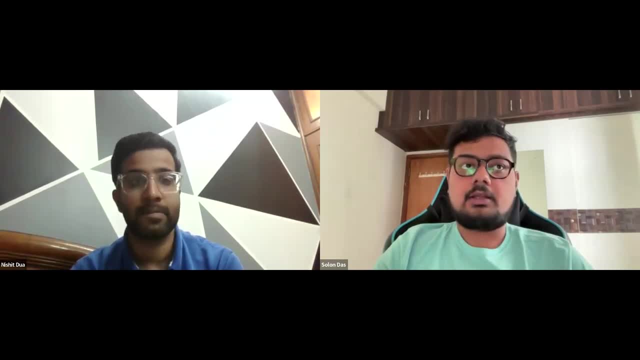 okay. okay, can you talk a little bit about memory management in spark? i haven't worked on the configuration side of spark. okay, no problem. so there are like few kinds of memories that allocates like you can go ahead with the like for spark. there is a reserved memory that takes like out of five gb, it would take three. 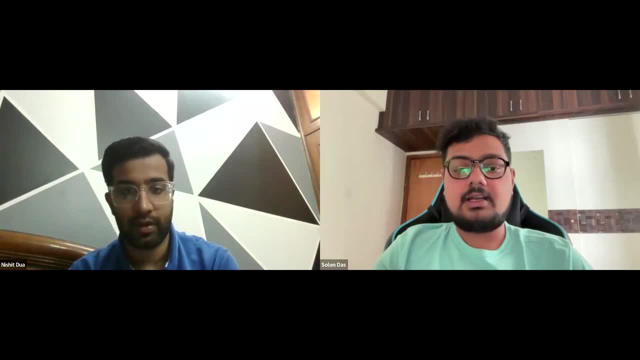 300 mb to the reserved memory. after that there is something called as overhead memory or the off-heap memory that would take around like. the formulation would be either maximum of 10 percent of the executor memory that you have requested for, or it would be 348 mb if that's not. 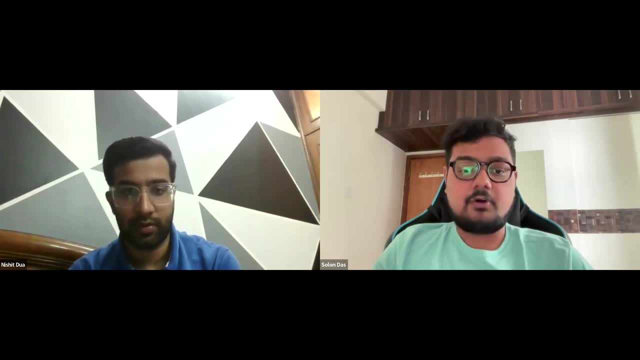 the maximum. the 10 percent is not the maximum, so it would be 348 mb. the rest of the memory that is left, it's divided into 60- 40 ratio. so within the 60- 40 ratio, 40 goes towards the operational levels and 60 is again divided into uh- 50- 50 in a ratio of 50, 50 out of which 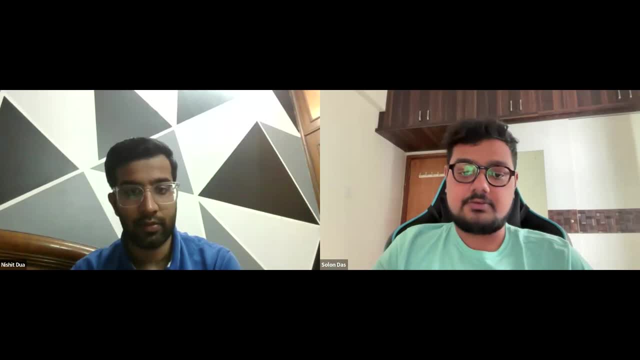 50 percent goes towards storage and 50 percent goes towards execution. now this 50- 50 percent could- uh, now there is a very thin line between these. like suppose you are caching a data frame or assisting a data frame and you need more than what 50 percent is there, so it would use up the 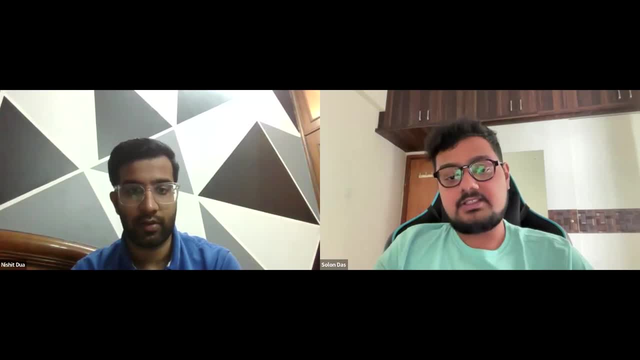 execution memory. in that case, and if you need a little bit more on the execution side, it would eat up something a little bit more of the storage side. this is how the memory is mapped inside when you uh request for a request for a memory to the executor. uh, no, worries, okay, let's move on to. 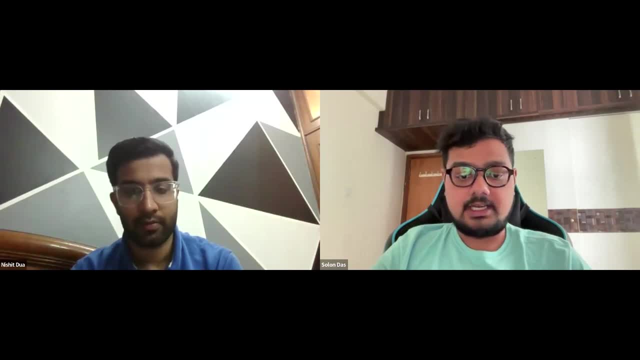 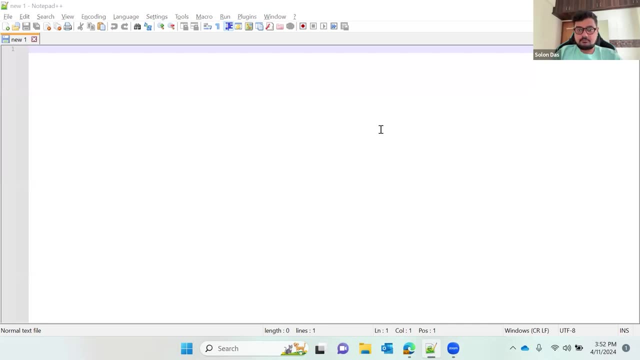 certain uh coding questions. i will share a link. uh copy the table first that i've pasted on the chat. got it right? so basically the table has it's a monthly sales table. it has two columns: month and sales amount. okay, clear, right. so every month: sales amount: what you need to calculate out of it is: 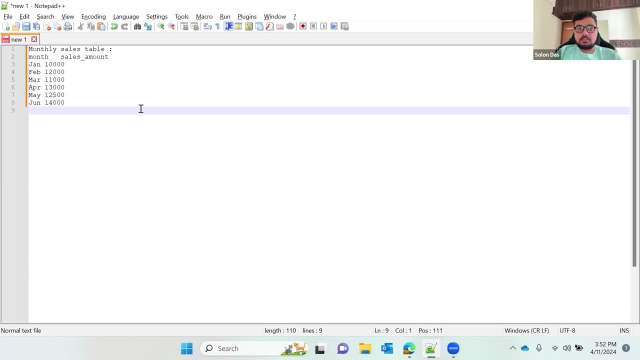 so i'm pasting the question, okay. so, uh, yeah, you can first page the question here. yes, so you need to calculate the difference in sales amount between each of this month, so the current month, and the previous month. Try writing this using a window function. Can you change the language to SQL on your notepad plus plus. 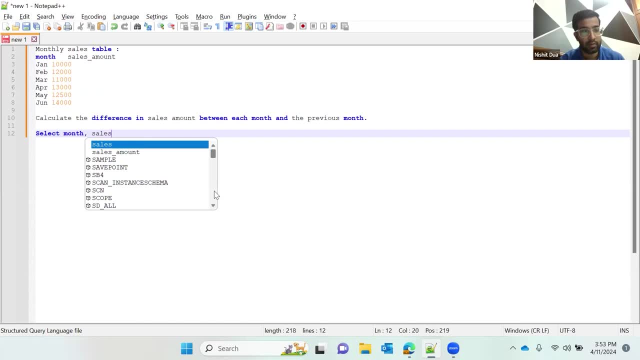 We want to calculate the difference in sales amount between each month and the previous month. So for this we can use lag and pass the sales amount. We want to partition it so we can just order by it on month column. 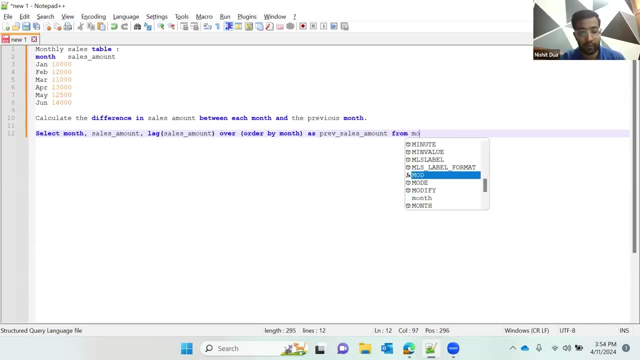 Oh, we're running out of time, sorry, Thank you, I guess this will work. Yes, for each month you can save someone by this previous sales month. Okay, works. 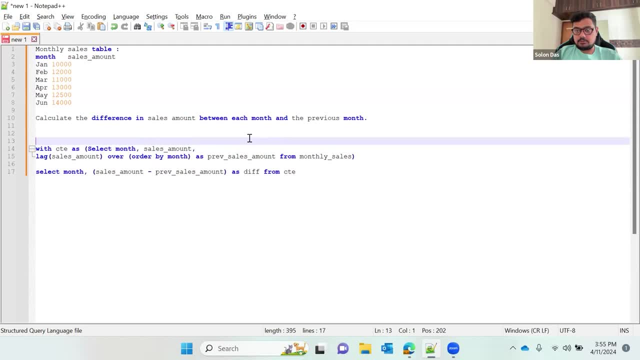 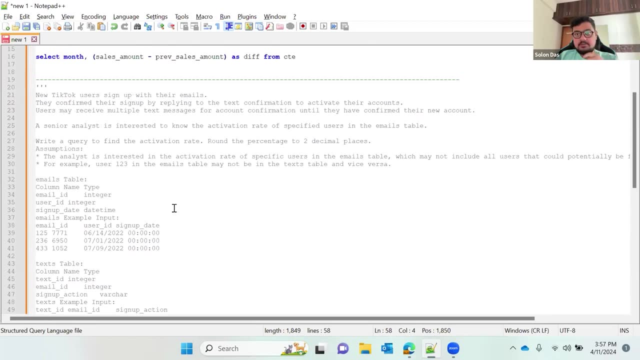 Cool, Let's move on to the next question. Sure, So yeah. so this is basically so. every so TikTok user sign up with their emails. So suppose any new user coming along is signing up with their email IDs and then they are getting a text confirmation out of it. 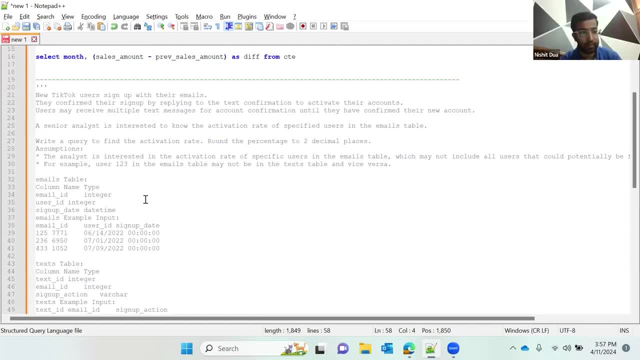 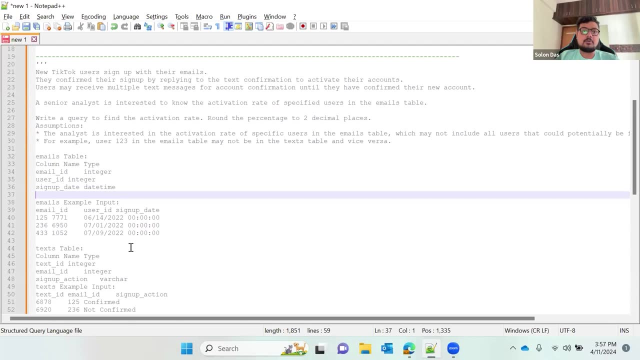 Now particularly, every user email can be associated with more than one Text confirmation. Suppose you get a OTP today and you did not actually confirm it, And again tomorrow you are coming along and giving another OTP, So your multiple text confirmation can come. 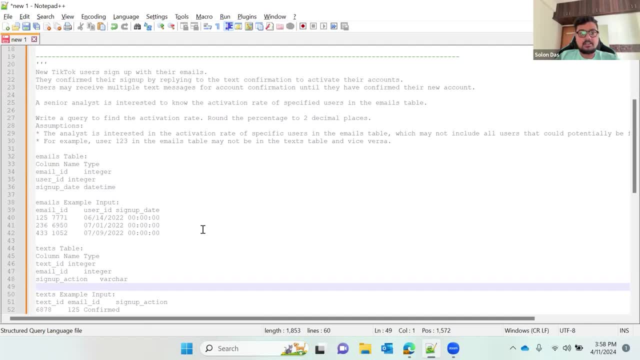 And, as an analyst, what you need to perform is you need to find the activation rate, like how many people are coming along, but how many people are confirming? what is the activation rate? Now, there are two assumptions to it. saying that an analyst that is interested in the activation rate, 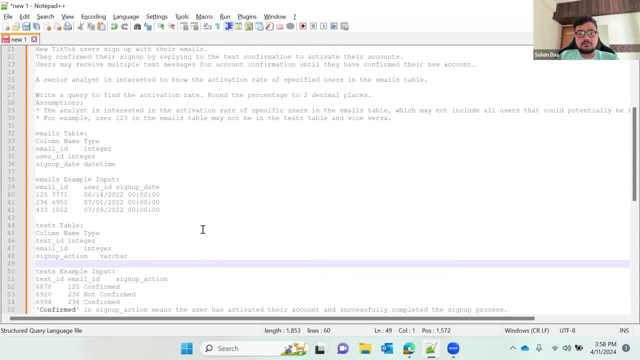 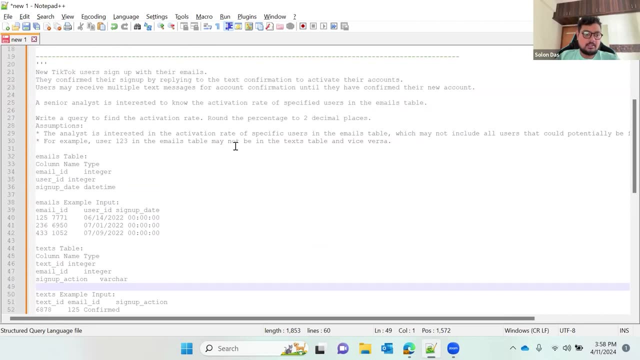 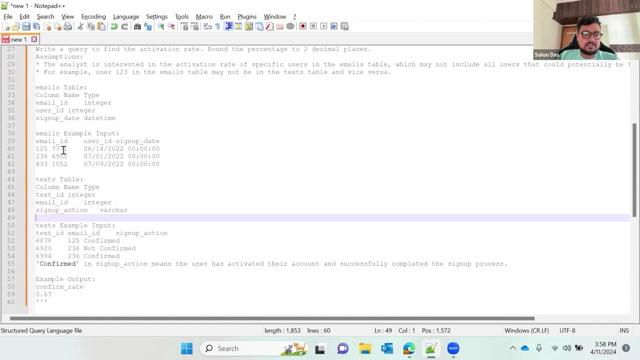 Okay, Okay, Okay, Okay. Okay. Email table may not include all the user that could potentially be in the email table, in the text table. So, like here, if you check the tables, like the examples, you see the email IDs, which is 1,, 2,, 5,, 2,, 3,, 6,, 4,, 3, 3.. 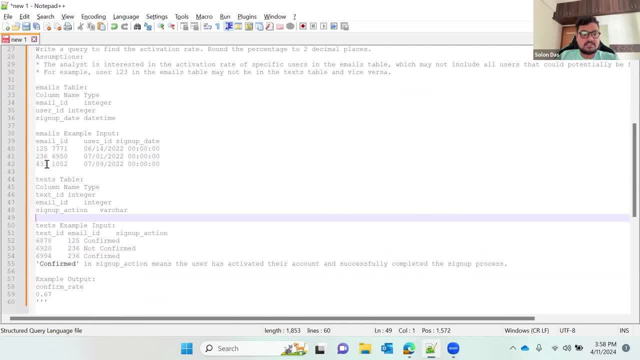 So 4,, 3, 3 is not present in the text table, Right? So this is someone who has, like, registered with an email but not verified his email. Okay, So this is someone who has registered with an email but not verified his email. 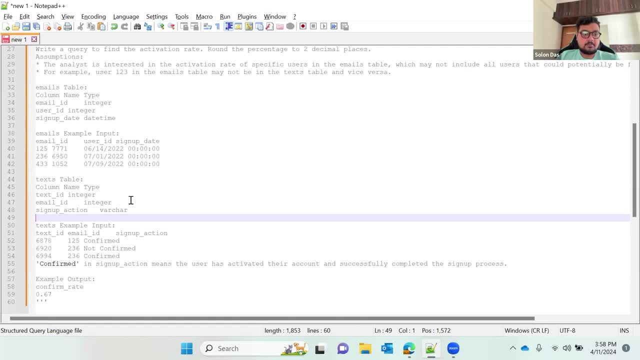 So this is someone who has registered with an email but not verified his email. Similarly, the other way around also might happen, Like, suppose there is a random 463 email ID that is present in the, like a text ID that is present, like 6996, that is present in the text table, which is not exactly present in the email table. 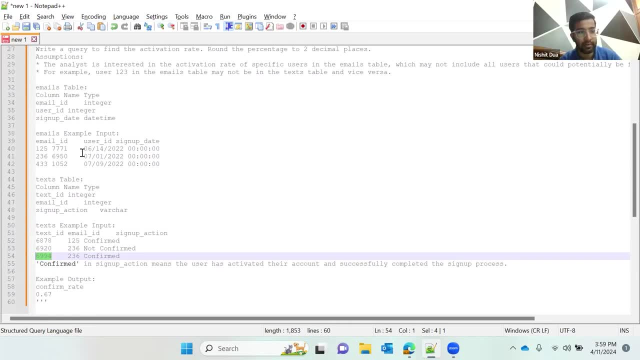 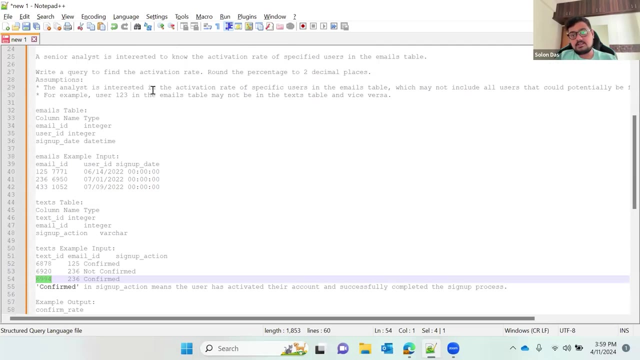 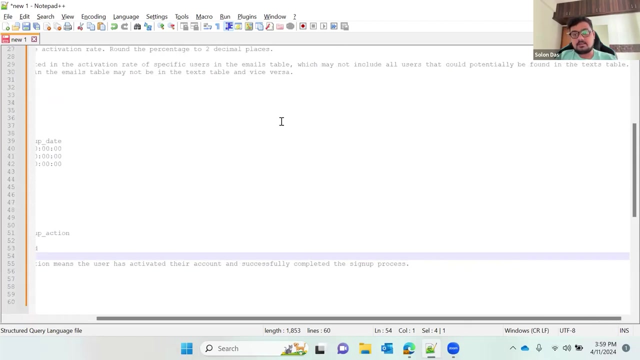 So? but we do not have any column for text ID in email table, right? No, I'm just telling you like it could happen. Okay, In this example- I mean that is the assumption- that is written, See the analyst. if you read the first point on the assumption, the analyst is interested in the activation rate of the specific user, which may not include all users that could potentially be found in the text table. 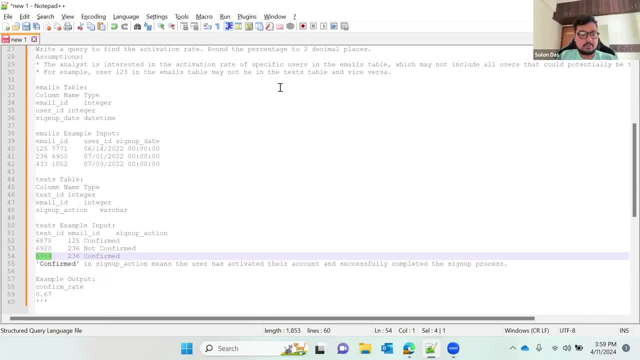 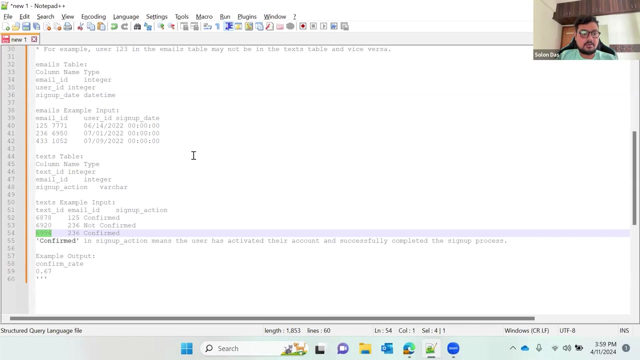 Okay, And confirmed signup action that you see confirmed. So confirmed is the signup action. That means the user has activated the account. Okay, Okay, Now what you need to find out is the confirmation rate. So suppose the 125, the email ID that you see 125, they have signed up on a specific date, which is the 6-14, so the June month. on the 14th of June that person has signed up. 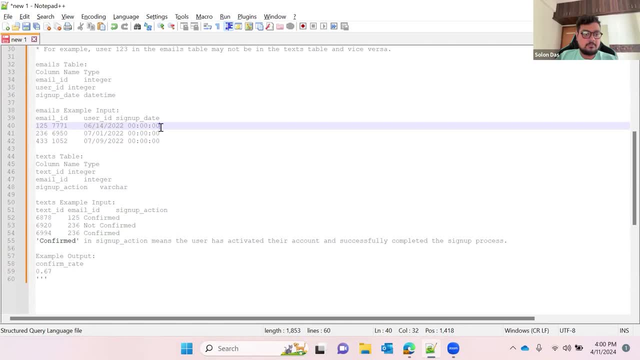 And then on 125, they have confirmed, but the 236, if you see, they have signed up on a specific date, but then on the first instance it was not confirmed and in the second instance it was confirmed right. 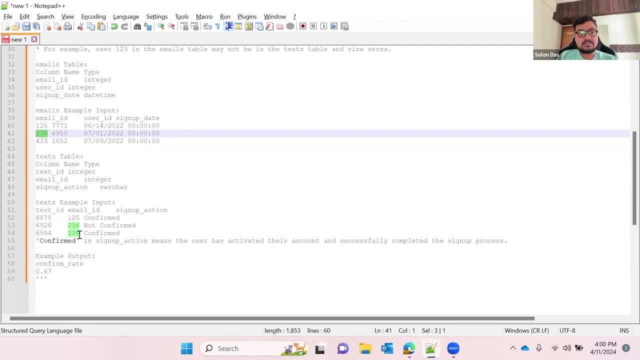 So 236 and 125 are two email IDs that were confirmed. So out of these three entries that you see, you get the confirmation rate, like 67% of the users. So out of these three entries that you see, you get the confirmation rate, like 67% of the users that are coming along are confirming. 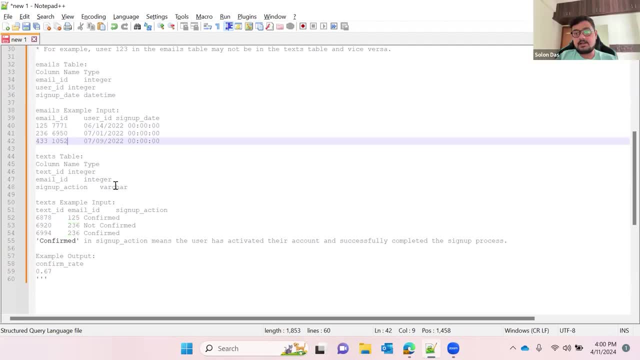 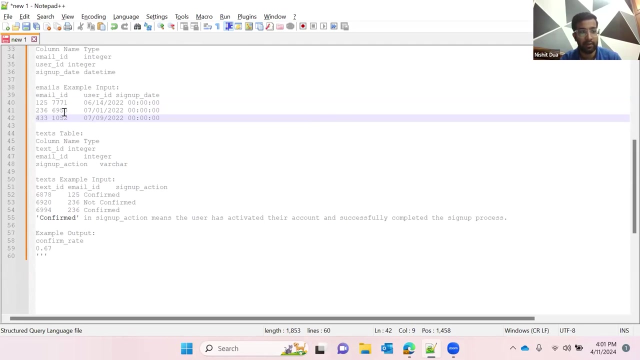 Okay, okay, got it. So the questions would be: write a query to find the activation rate. round the percentage to two decimal places. Sure, Okay. So the total user IDs are 7771, 6950, 1052.. 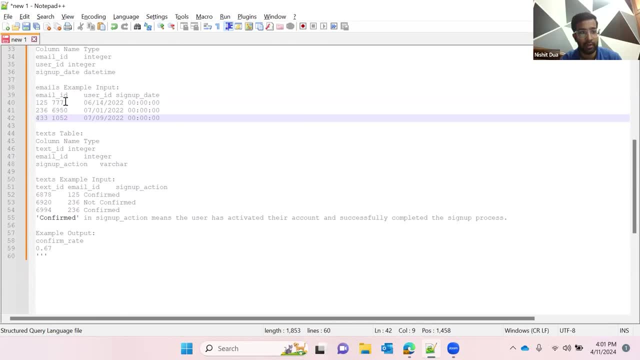 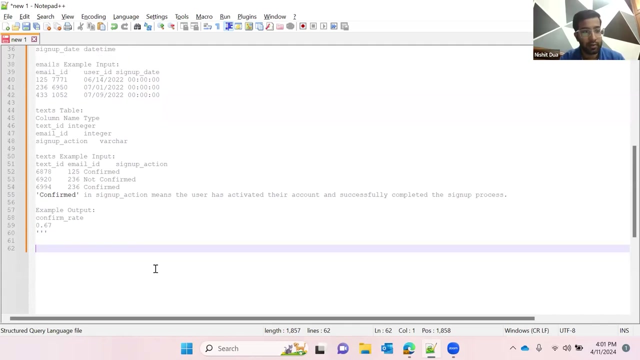 Out of these three two confirmed which were having email ID 125 and 236.. So out of these three, two confirmed which were having email ID 125 and 236.. Yeah, okay, So first we can just filter out the confirmed action in the text table. 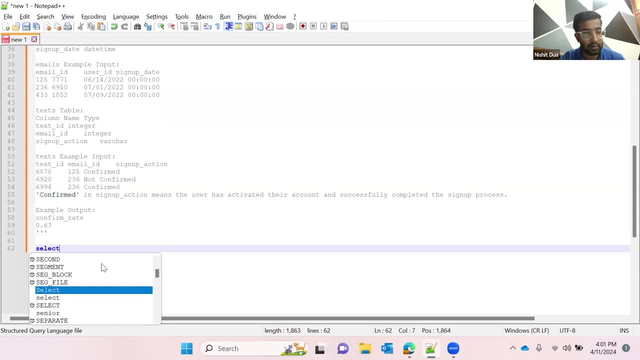 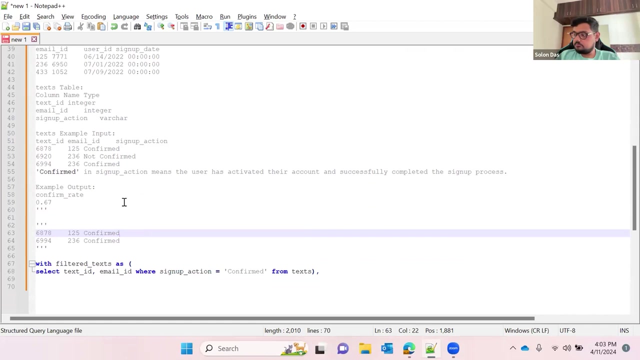 Okay And Okay, Thank you. We'll get these two cards Again, So you can now. We'll get these two cards. We'll get these two cards, So you can now. This is, I'll name it. 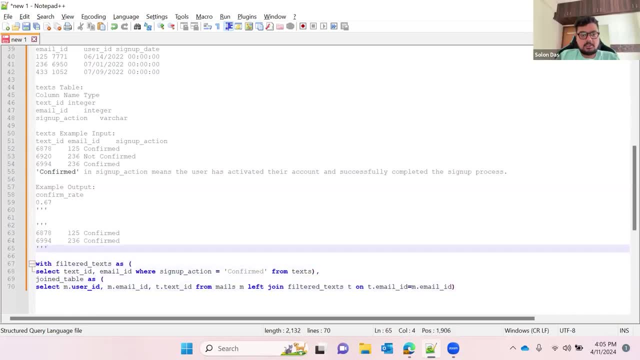 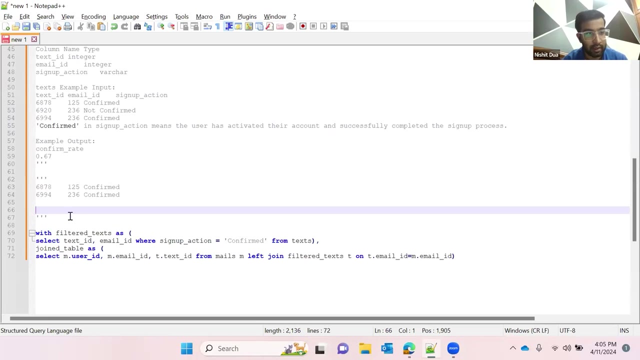 So at this Join table that has- And you have the tables- one email id picking up user id, email id and text id. okay, so at this step we will be getting output as: uh, text id would be six, eight, seven, eight, one, twenty, sorry, sorry, we are having. 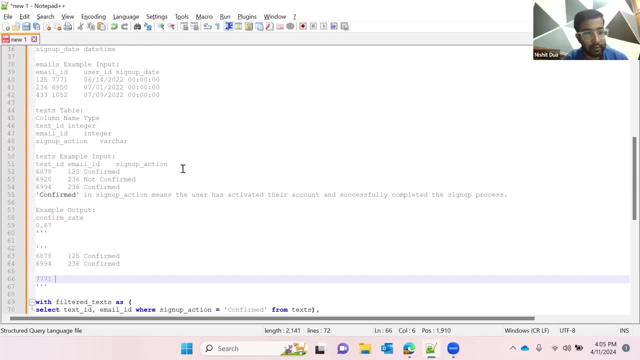 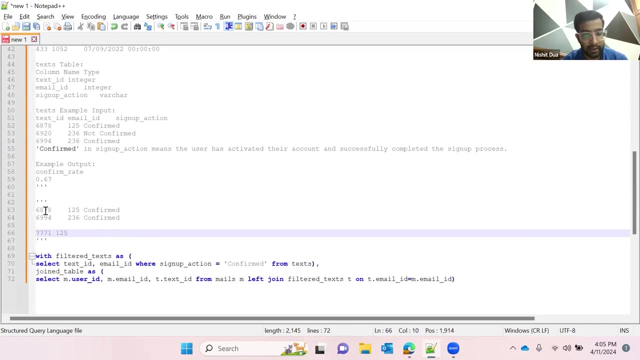 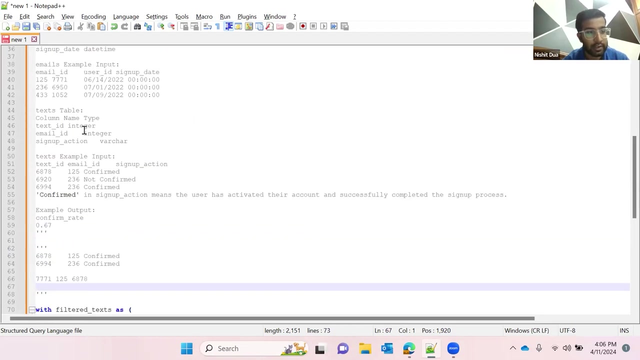 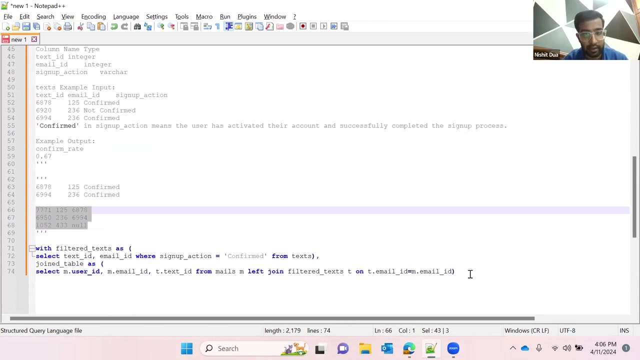 seven, seven, seven, one having email id as one to five. text id we have as six, eight, seven, eight is zero. so at this point we get this output and again then we can see it. so x id, or do we want percentage or uh, first out, but no, okay. 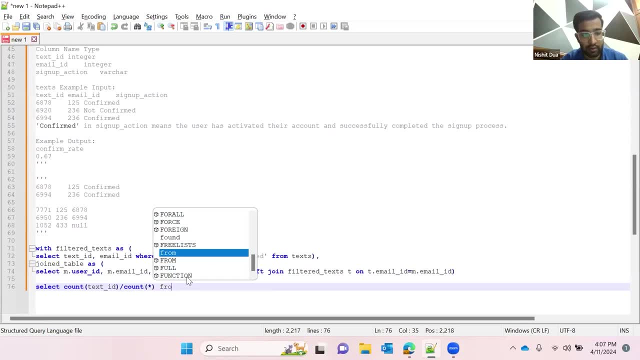 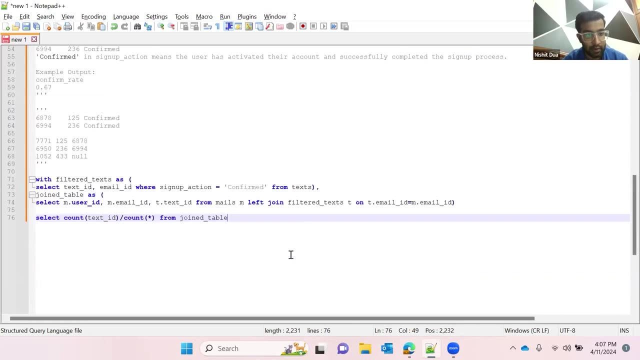 uh, let's see. okay. so here count star would be three and count text id would be two, so it would be returning us point six, six. we can also round it to two decimal places. i guess this would work. yeah, Yeah, this would work Perfect. But I think the count that when you do a divide you can. 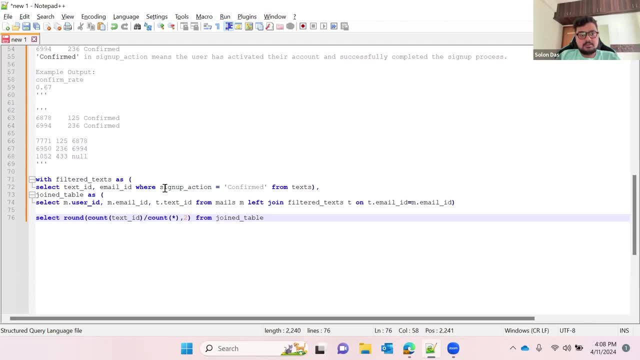 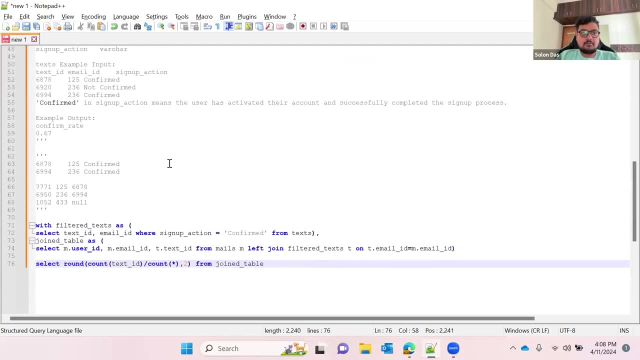 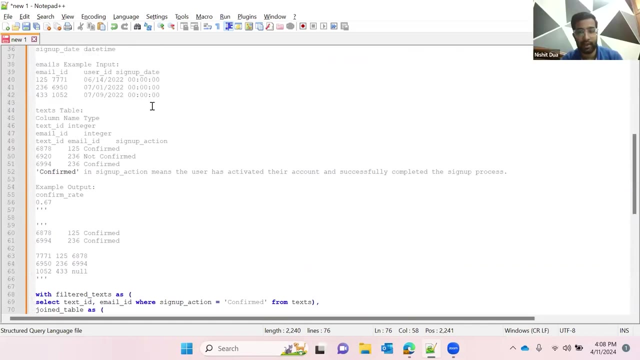 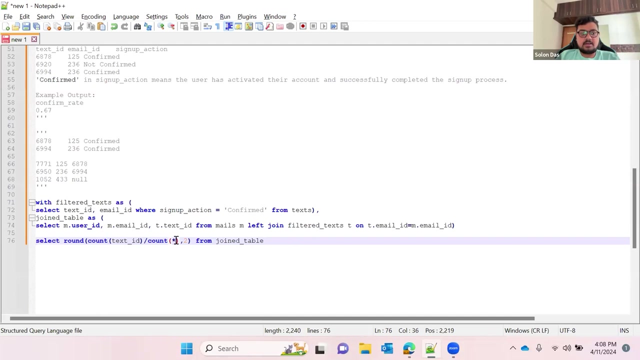 do a count by distinct email ID? Why? Because a count star there, if at all. email ID is repeating in future, So that would count star all the email IDs, even if a duplicate email is present. So can a different email ID be present? Yeah, it can be, Suppose someone is trying, So you. 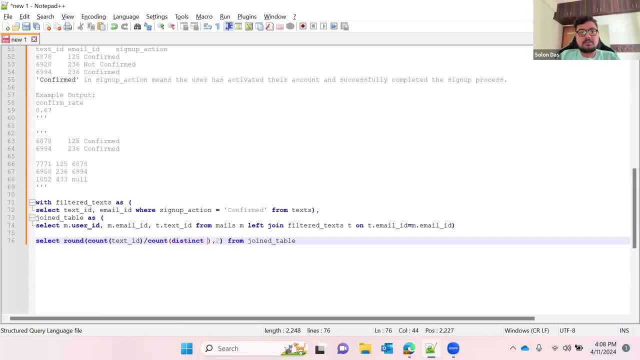 must have also faced this right. When you go to sign up, sometimes you do use the same email ID again and then it basically tells you you have already used this email ID, So that gets registered, but then no confirmation comes out of that because you never use it. 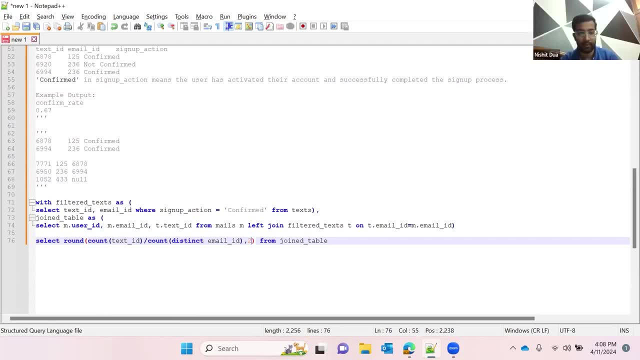 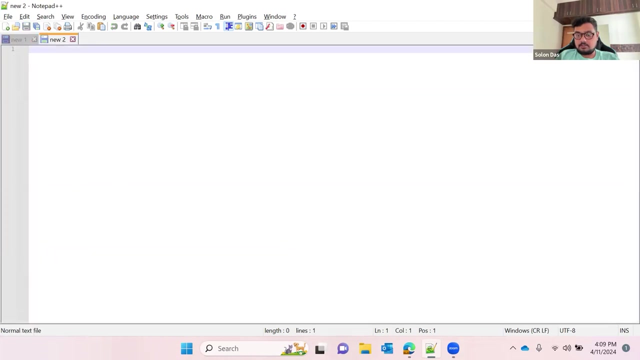 again. Okay, So it would be a distinct email ID here. No, it's completely correct, Okay, Great. Okay, You are comfortable with normal Python, right? Yeah, Okay, Let's do this question So straightforward, simple question. I'm pasting it on chat. 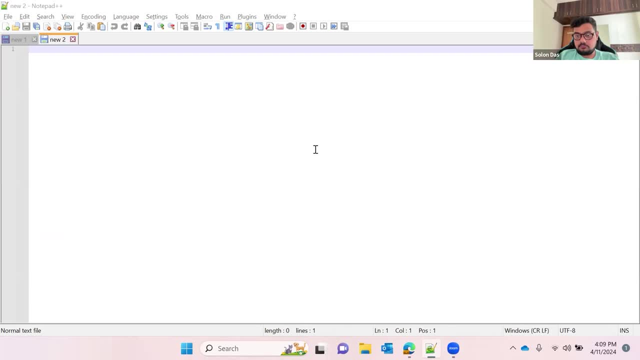 What can you see? So there is just assumption here, not assumption, basically a constraint here. You can copy the constraint also. Yes, it's the same. Okay, I see, Okay, Okay. so, simply, you have a list of elements here: 0, 1, 0, 3, 12. okay, now what we? what we need to do is: 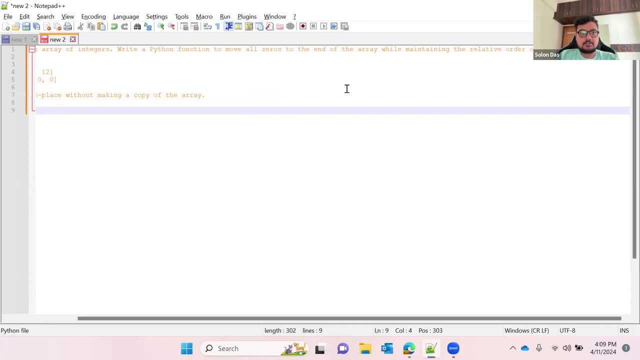 write a function like a define, a python function that would take in this list and it pushes the zero zero elements to the right side and pushes all the non-zero elements to the left side, but then you don't change the relative order of the non-zero elements. basically, you don't sort it. 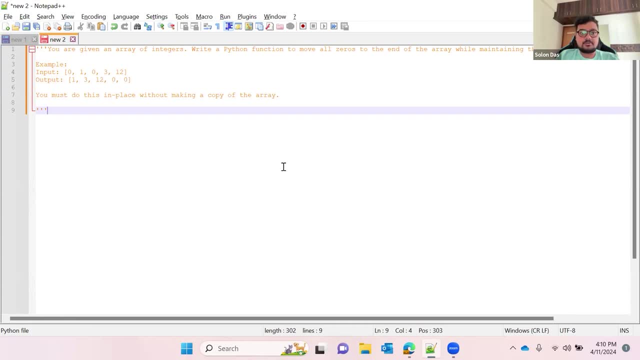 because if you sorted, this kind of problem solves itself. right, but you don't have to sort it, but you have to move the non-zero elements to the left side and zero element to the right side. okay, okay, and the constraint is you don't use any extra space or any extra data structures for that. 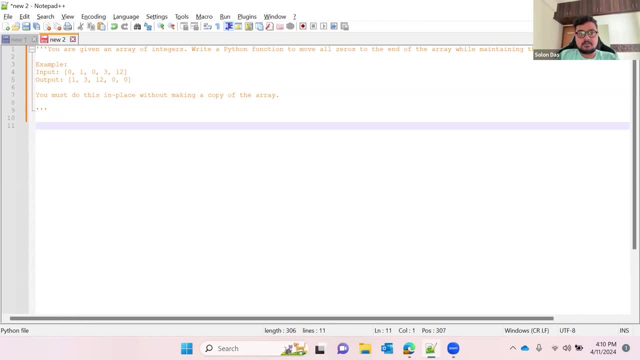 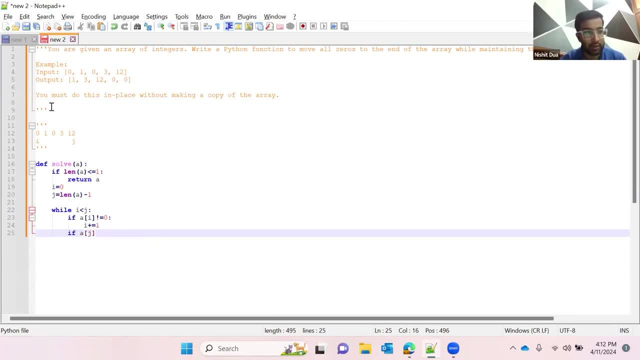 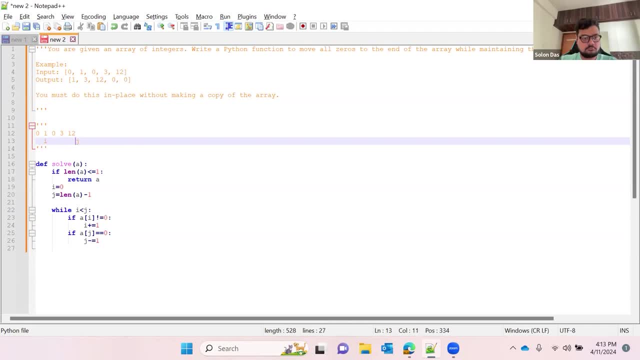 so, move, keep incrementing that one, and j is also not zero, so j will be here only. so if it is not zero, then it would, so i would be here only, j will also be here, and if a of i is equal to zero, in this case, it would replace: oh, okay, okay, but we should be. 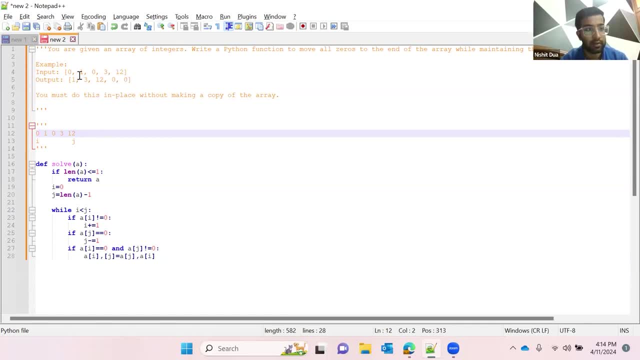 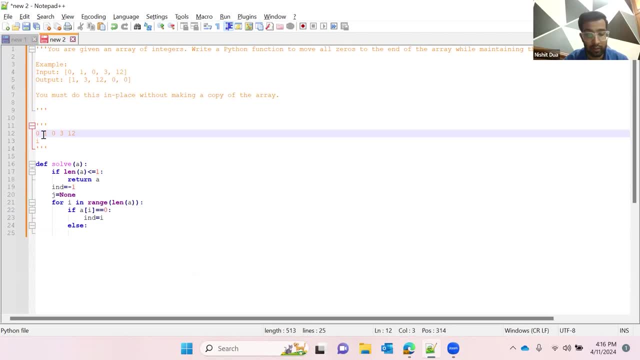 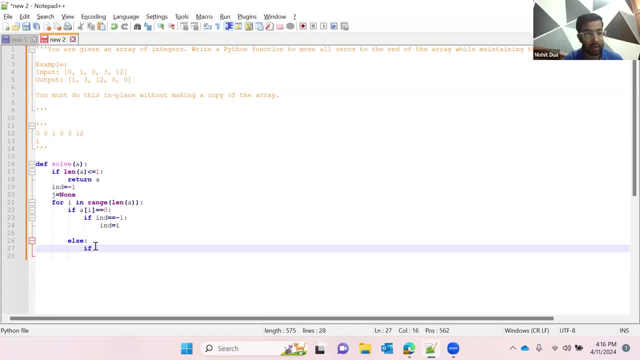 It would be mapped to the first 0 in our list. And let's say, if we encounter a non-0 element, So, and if our index is not minus 1, then we can. index is not minus 1,, then we can. 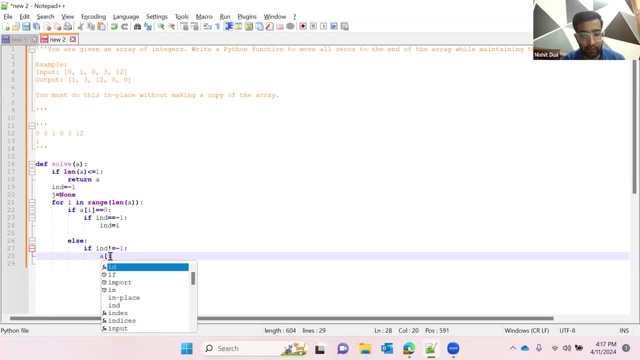 replace the index with 0 here, and then we can replace the index with 0 here, and then we can replace the index with 0 here, and then we can replace the index with 0 here. Thank you, Thank you, okay, no issue, we will just move to the next question, as we have like 10 minutes left, so 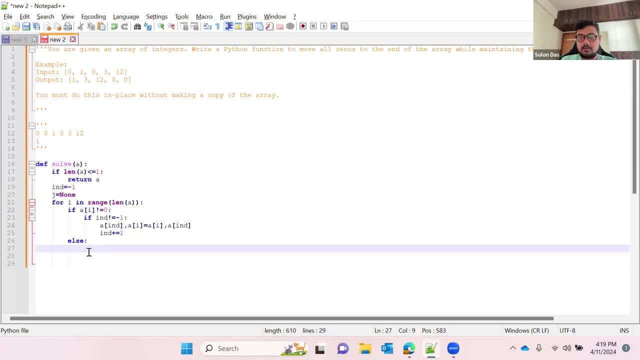 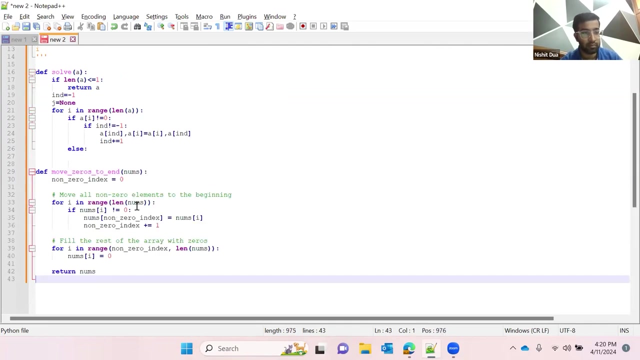 uh, we move on. i'll just uh paste the answer here. uh, ideal answer here, so that everyone can see. can you paste this uh to your? sorry, i did not paste uh, just a minute. yep, can you paste this on the notepad, okay? so basically, what we are trying to do is we are trying to shift the non-zero elements to the left. 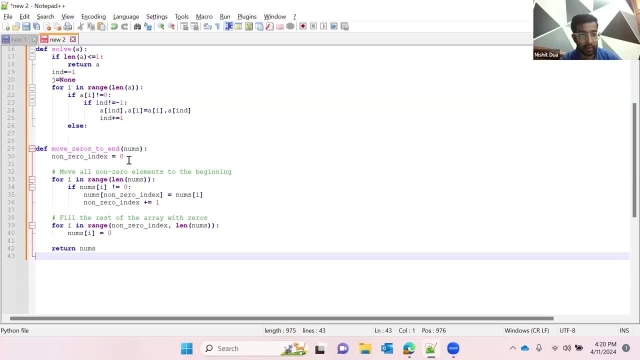 and the zero elements to the right right here. uh, so we are catching a non-zero index which starts with zero. you started right- i mean the first approach that you started with right- the you started indices as zero, which which was right. then you basically loop over all the elements. 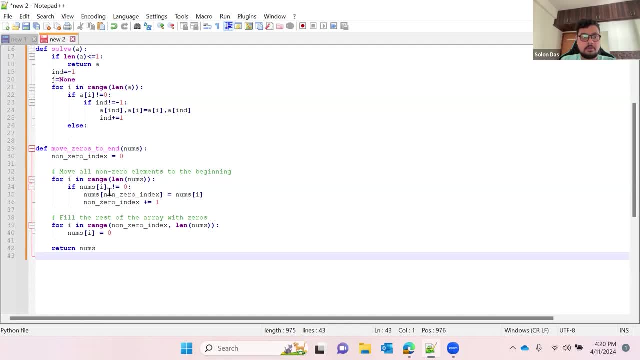 and you find out whatever is not zero. basically, you do a nums of non-zero index, so the zeroth index will be replaced by the specific element, and then you increase the non-zero index by one. in that sense it will go on like zero and for for every zeroth index that. 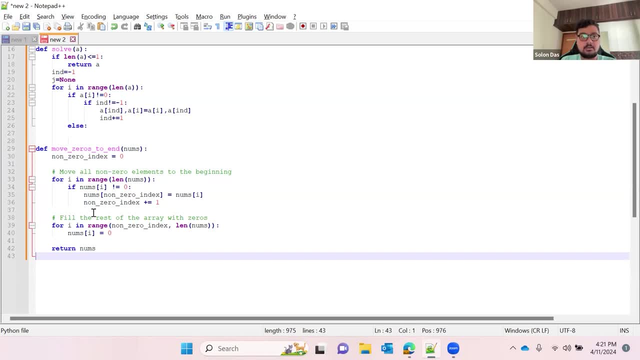 is coming. it won't increase the non-zero index to one right by one. it won't increase. so for the second index, it would give out one and two, or after your non-zero elements are in place, what you need to do is run a loop from your last of the non-zero index. 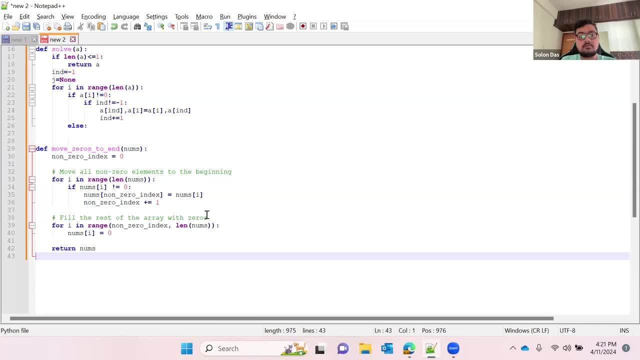 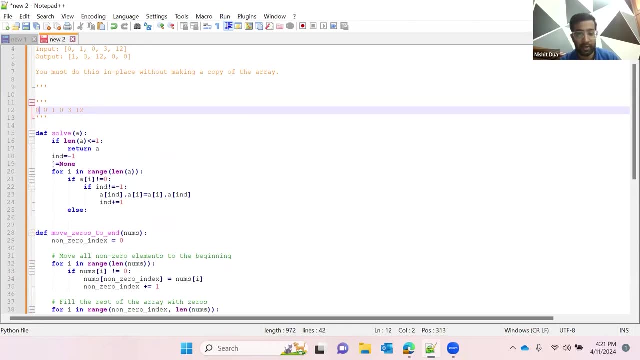 that you have, suppose, your three to the length of nums and you build zero in it. so in that sense you will replace. so in this case it would be replaced by one. yes, the zero would be replaced by three, twelve and twelve and, uh, in the last loop, all these three would be replaced by zero. 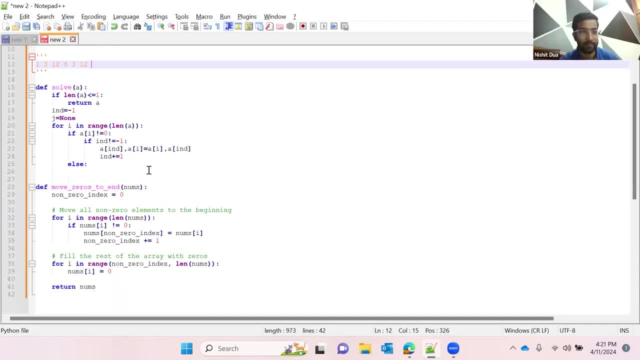 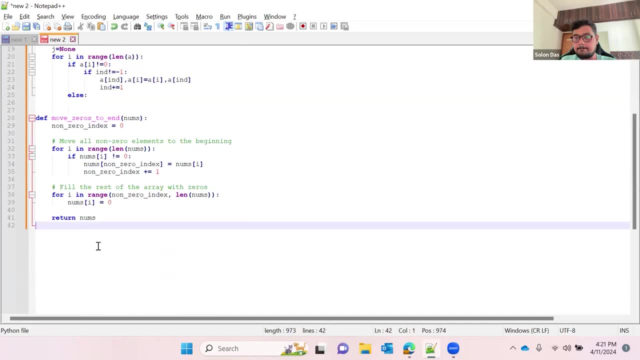 by zero. yes, okay, okay, okay, no issue. uh, let's move on quickly to the next question. okay, uh, let's see if we can do this. okay, can you paste the question and the example on the notepad? this is also. you need to do it in the same array itself. 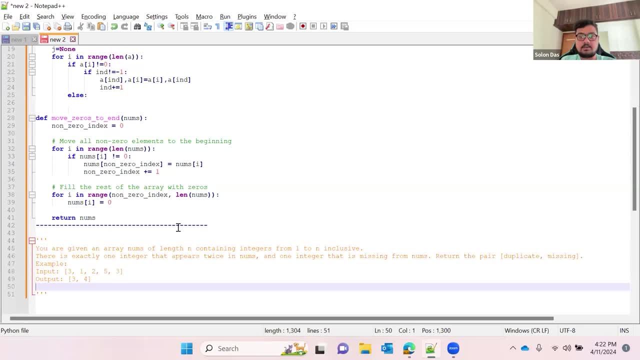 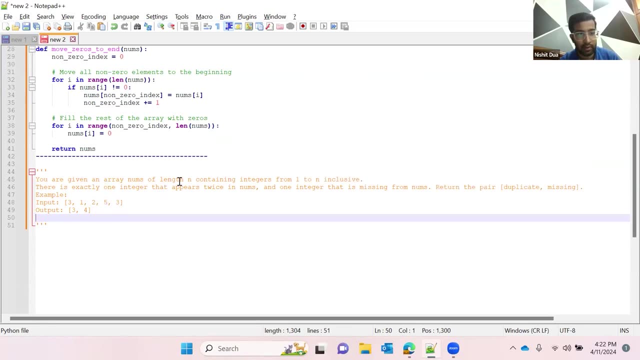 or you can try doing it using another array, if that is easier, and then, if we have time, we can optimize it. sure, so you're doing an array, so you are given an array- three, one, two, five, three, suppose. so all the inclusive elements from one to five. is there what you have? to find out? what element. 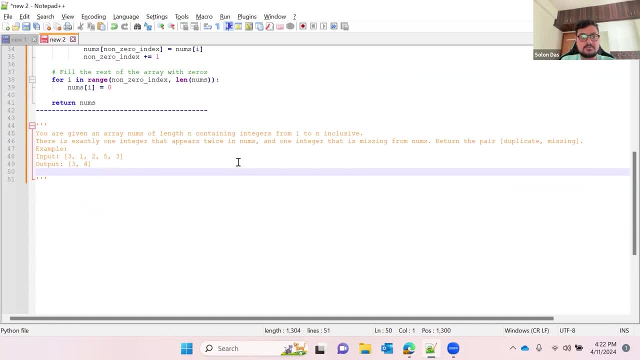 is repeating itself. so suppose three is the duplicate here that comes first. so you have, your output would be a list of duplicate comma missing and what is missing between one to five. so four is missing, right, okay, okay, yeah, that's the question. so i mean, just like there would. 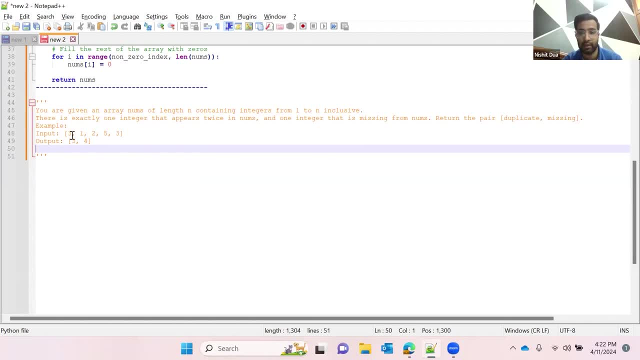 be only one, uh, which would be uh extra. yeah, like, suppose it's a 1 to 10, like this is one of the examples. it it could work with any use case as such. yes, this 1 to 10, and out of that 2, 5, 5. this is visible, complete, so that's the immediate solution. yes, it is. 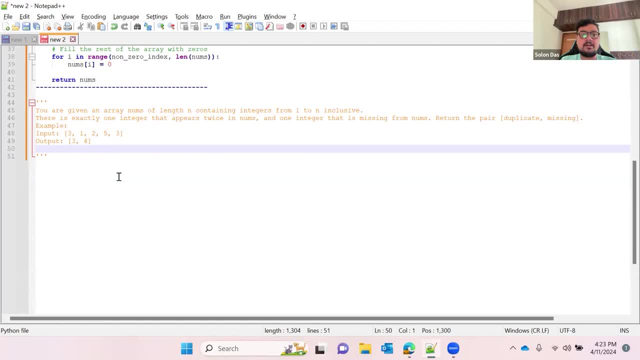 one to ten and out of that 1 to 15 is theRel��TodaySansung videos. so we can find out what is the number one and is the number two and is the straight number. two, five, six might be duplicating itself, so you can pass on like two, five, eight. first. 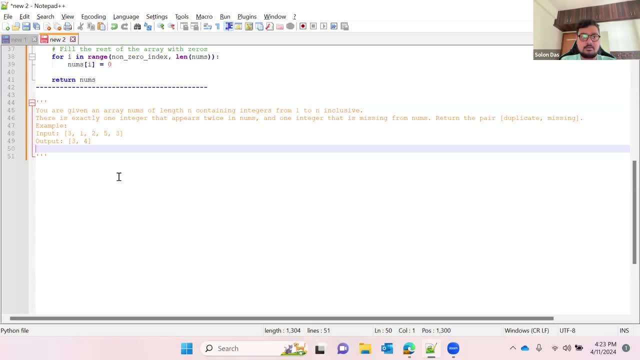 and then comma. suppose nine is missing, then you can pass on nine, so like that. oh, can you paste this example too? suppose let me paste it. suppose your input is. so suppose two numbers are missing, so suppose this is your input. your question says there is exactly one integer that appears twice in nums and one integer 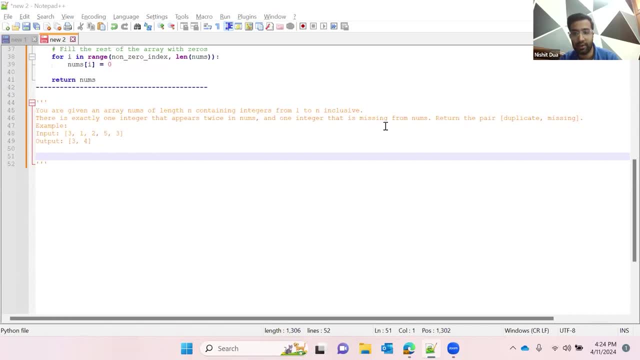 that is missing from nums. so that, yeah, i mean in this example it is. i mean here there is exactly one integer, that is three, three. suppose you have two integers. i'm saying i mean just to kind of add a layer onto it, onto the question. suppose you have two integers, suppose 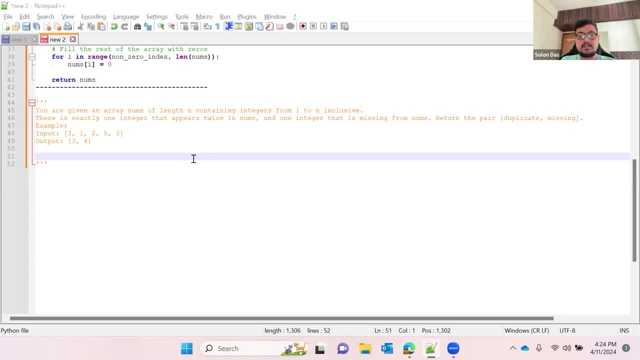 six and seven. these, these are two integers that are repeating itself. you can pass a list to that so your output will look basically a list in list. right, there would be two lists so it could say six, seven are duplicating and eight and eight and nine are. 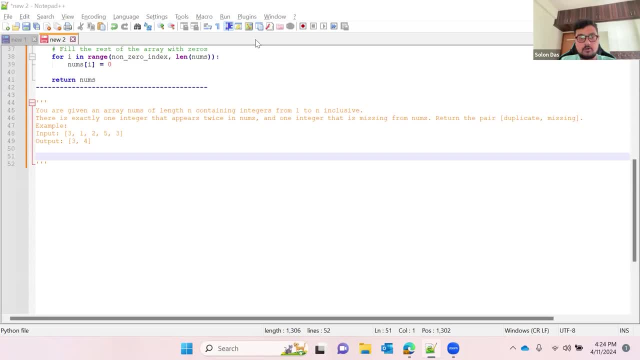 missing. so this could be the output. you can copy the input and output here. i'll just clarify that. okay, suppose it's a number from one to ten. okay, here you see, six and seven are duplicating. so in the first place. so in the master list the first. 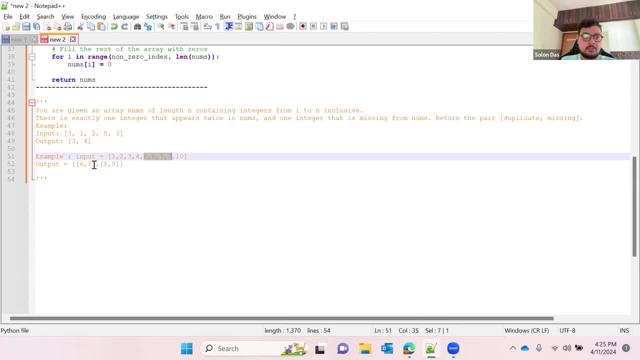 i of zero would be six, seven, which will have j zero and j one, and then in the next i of one you will have the missing element, which will be again j zero and j one. so eight and nine are missing and six and seven are missing. so again, if this is a little bit difficult layer for you, you can go. 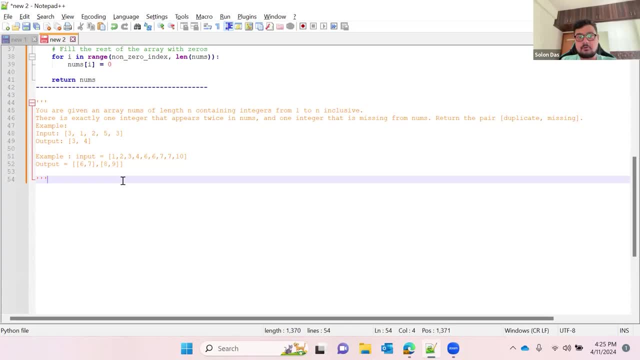 forward and solve the first layer first, then we can look, look towards this. oh sure, so in this case, uh, if only one number is being repeated and one number is missing, then we can, uh, just take in zor of the whole array. so in this case, the czar would be: and also: 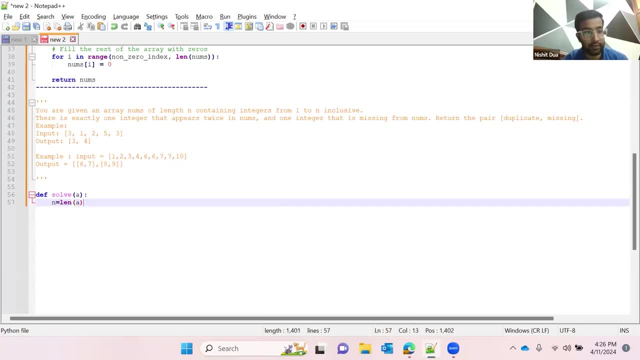 so let's say we're five, so you so here. we will get put as so at this step. x would be holding zor of three and four and four, and that's one of the otherwise like theuzor operator. those four is missing, four is being taken and j is missing here. 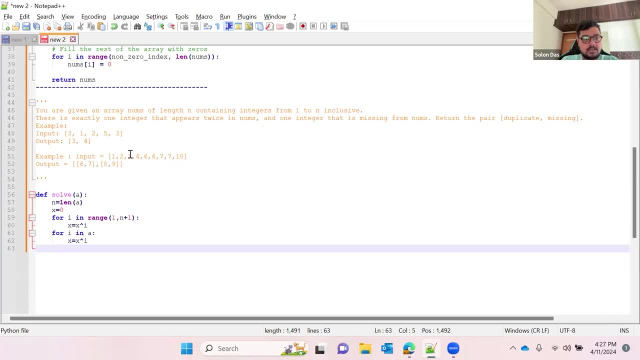 so. so before you go through this approach, can you also explain md1 like: uh, how does z pawn operator works? i think that would like what is like the operation behind zor operator, like: suppose it's a similar character, like x or x, what would it give? and x or x 0, what would it give? 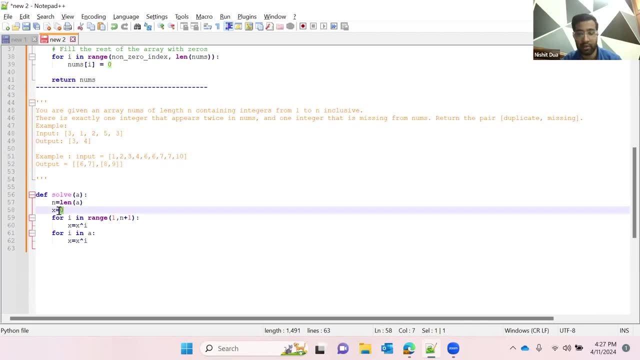 so i stand c nor, but it or does this works? x started with x0, so any number is or to zero, it would be resulting in the same number. so if we is, or like, let's say, in this array, if we are taking sort of three comma, three and three, 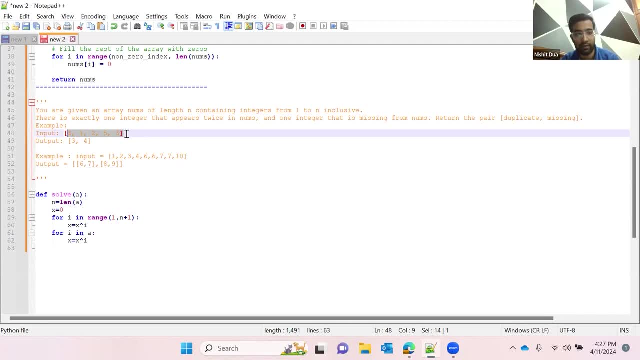 it would result in zero, so it would like uh. we can get which uh number is has been duplicated, so like similar. in this case, if is all six, six, and then seven, seven, and a total door for this array would also be zero. so for this number, for this array, we are taking xor from all the 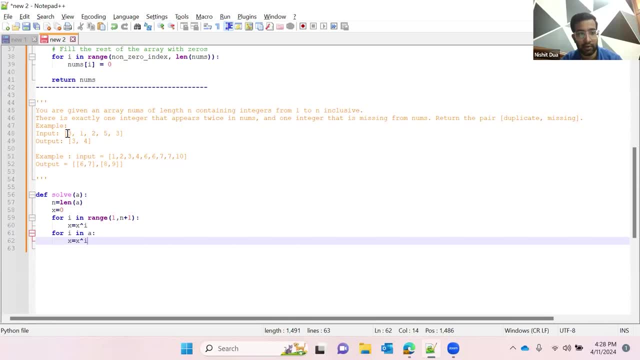 elements from one to n, then taking xor on this array or list, so the resulting would be xor of 3 and 4.. now we can so in your line number 59 and 60. so the syntax that you have written for i in range of 1 to n plus 1. 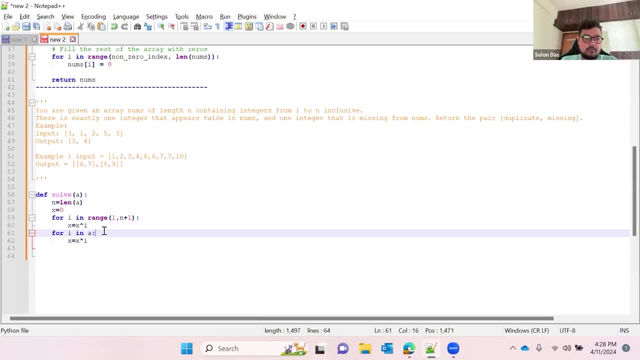 so in the last index i think it would go out in a out of index error because it would go to search for a n plus 1 index. it is an index and not the area of index. sorry, i'm not passing the a of i, i'm just passing the index like it is. 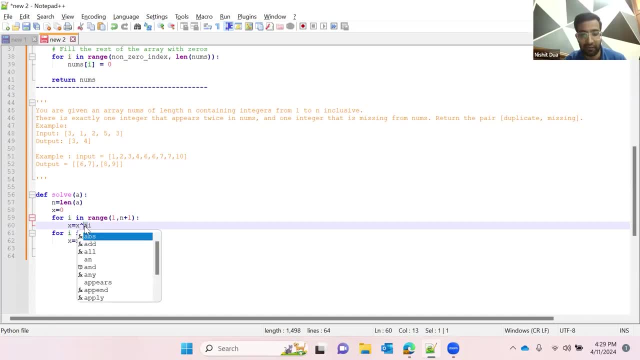 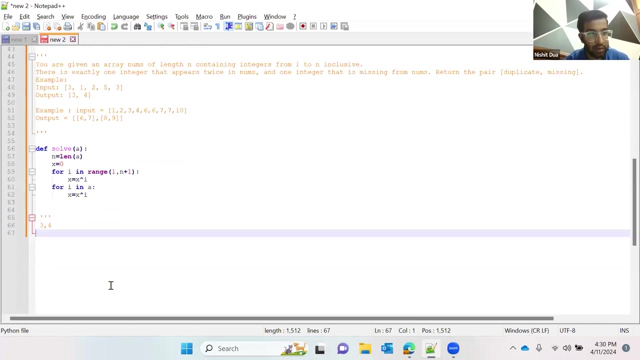 numbers from 1 to 5.. i'm not passing the a of i. if i would be passing a of i then it would been gone out of index. here i ranges from 1 to 5, so we can just take software. so you. 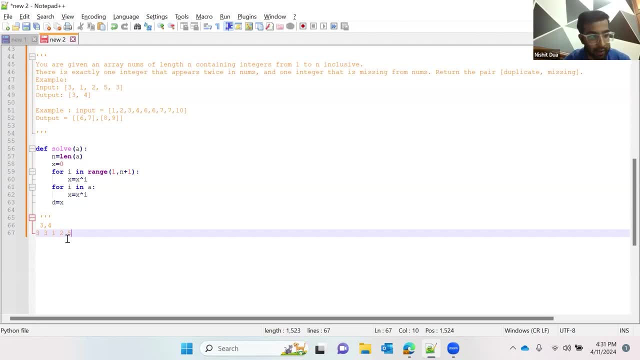 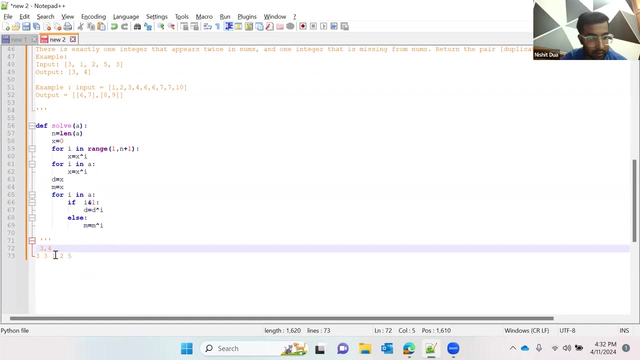